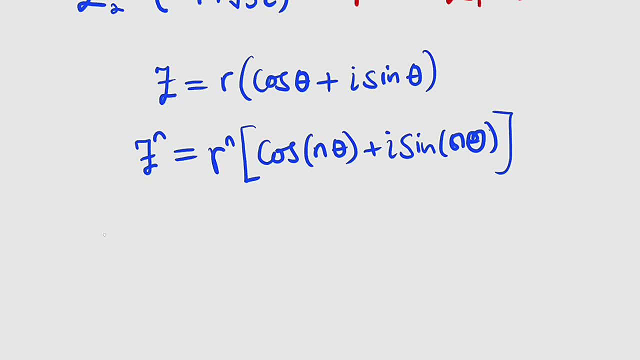 have two complex numbers, z1 and z2. z1 to the power of n, for instance, this is the same thing as r1 to the power of n, then multiplied by cosine of theta 1 multiplied by n, or n multiplied by theta One is the same thing then, plus i sine of theta 1 multiplied by n. then for z2, suppose we have: 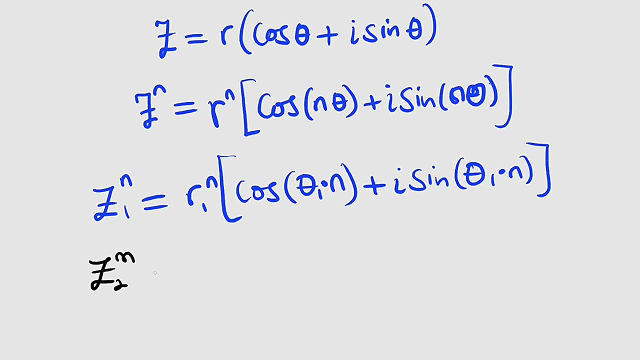 another one, z2, raise to the power of m. this time around this is equal to r 2 to the power of m, then multiplied by cosine of theta 2, the multiplied by m, then plus i sine of theta 2 multiplied by m. So this is for the second complex number. So what? 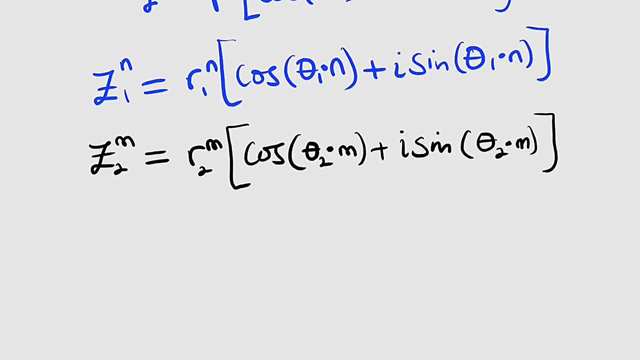 if we wish to multiply these two complex numbers together, Suppose we want to multiply z1 to the power of n, then multiply by z2 to the power of m. This is the same thing as r1 to the power of n, then multiplied by r2 to the power of m, then multiplied by cosine of what. 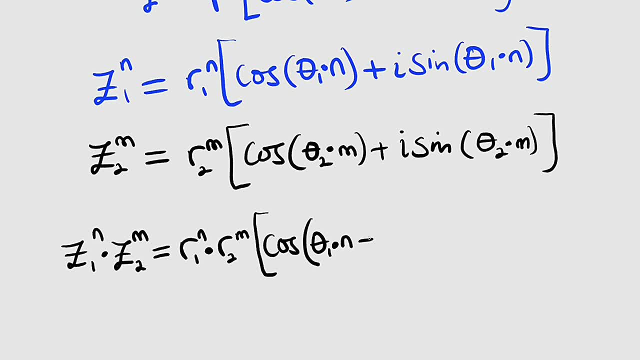 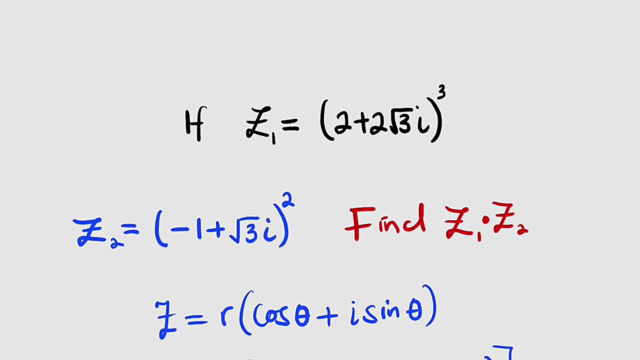 multiplied by n, then plus, then plus i sine of, multiplied by n plus theta 2, multiplied by m. So, finally, this is the equation we are going to apply in multiplying these two complex numbers together, And hence we are going to transform each complex number here into its polar form. 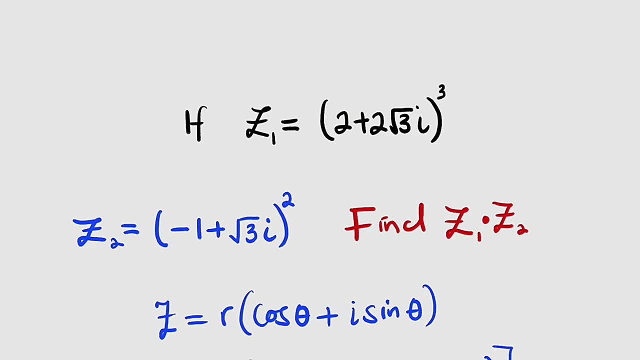 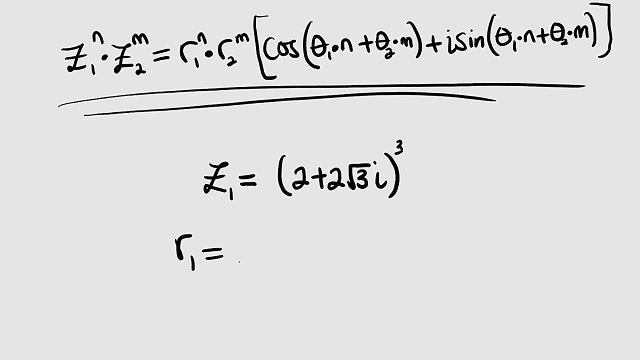 Then we raise it to its power. Let's start with the first one. So this is our first complex number. Let us find R1, which is the modulus. This is equal to the square root of the real part squared, which is 2 squared. 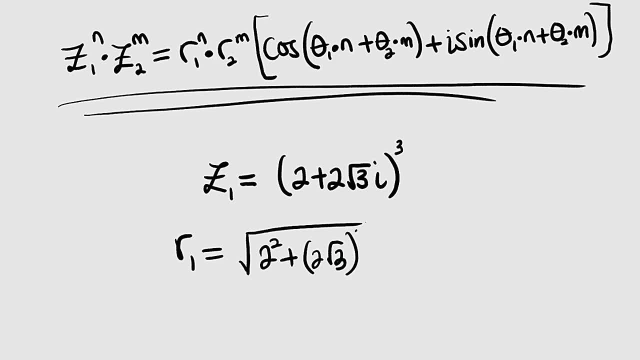 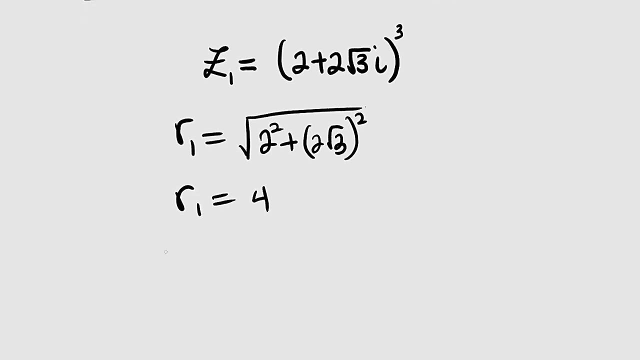 plus the imaginary part also squared, This is 4, and this is 12.. If you add them together, you have 16.. The square root of 16 is 4.. Therefore, R1 is equal to 4.. Then what about theta 1?? 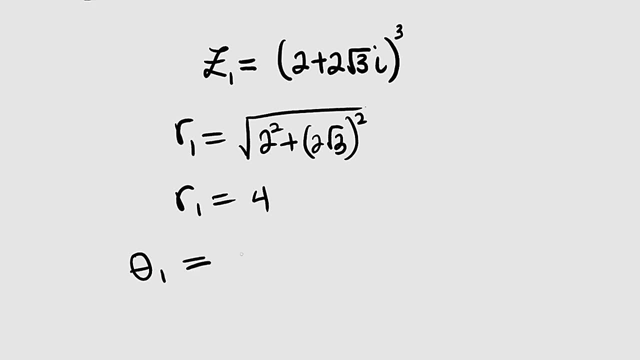 Theta 1,. this is equal to tan inverse of the imaginary part, which is 2 root 3, then divided by the real part, which is 2.. 2 root 3 divided by 2 is just root 3.. And what is tan inverse of root 3?? 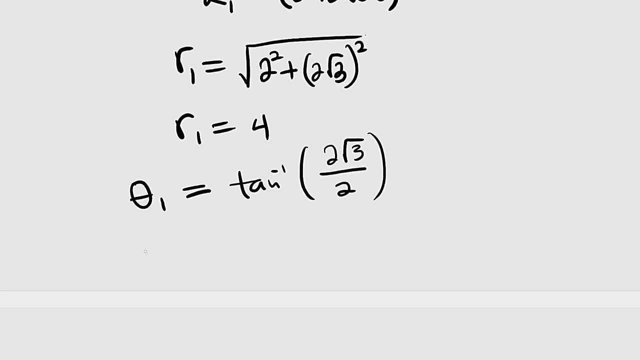 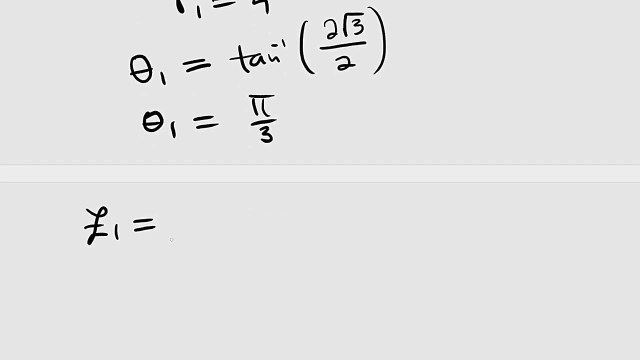 It's pi divided by 3.. And therefore theta 1 is equal to pi divided by 3.. So what is the polar form of this complex number Z1.. Remember, it is R1.. R1 is 4.. Then 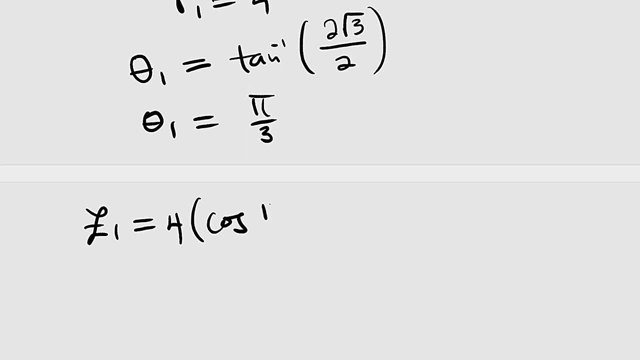 multiply by cosine of that angle which we have as pi divided by 3.. Then plus i sine of the same angle, pi divided by 3.. But remember, our complex number is to which power? To the power of 3.. 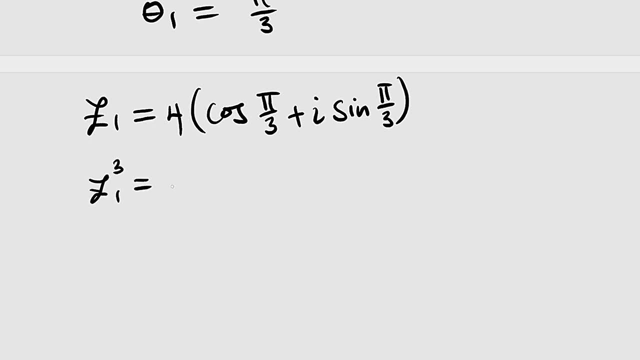 Therefore, Z1 to the power of 3 will be equal to 4 to the power of 3.. Then multiply by cosine of what 3 multiplied by pi divided by 3.. Then plus i sine of what 3 multiplied by pi. 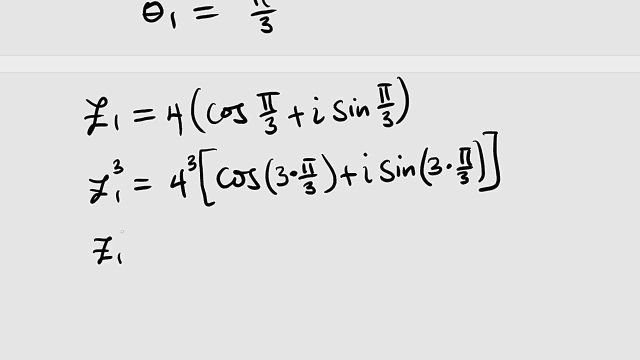 divided by 3. Z1 to the power of 3 is equal to 4 to the power of 3,, which is 64. Then multiply by cosine of pi, because 3 will cancel 3, plus i sine of 5.. 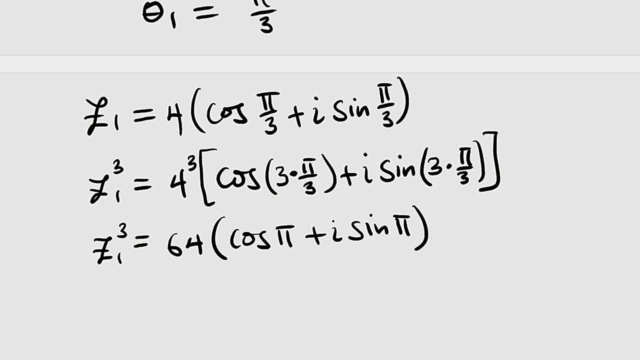 So what I have done with the first complex number, Let us take the second one. The first complex number, Let us take the second one. The second complex number is negative: 1 plus root 3i to the power of 2.. 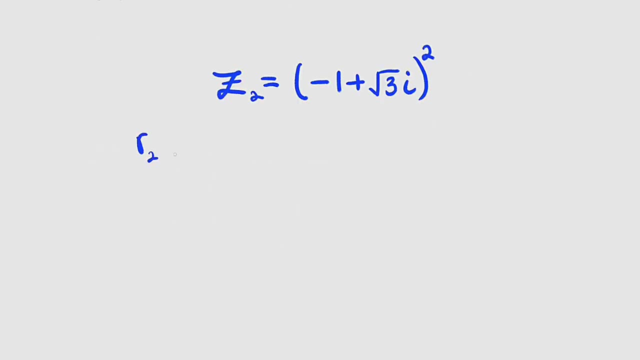 So here is our second complex number. Let us find R2, which is the modulus square root of negative 1, squared plus root 3, also squared, This is 1,, this is 3,. 1 plus 3 is 4,. 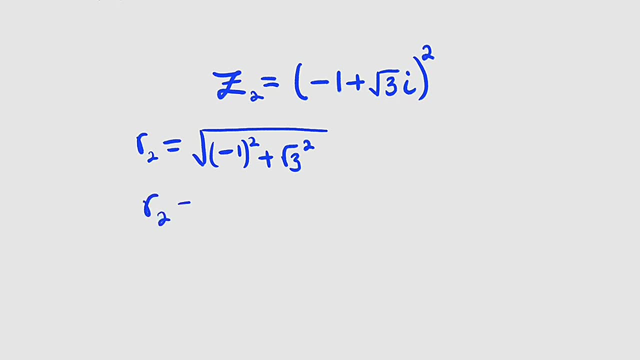 square root of 4 is 2.. Therefore, our modulus for this complex number is equal to 2.. And what about our theta? It is equal to: if you observe, this is in the second quadrant, which is less than 180.. So we are going to let assume we are in the first quadrant using that. 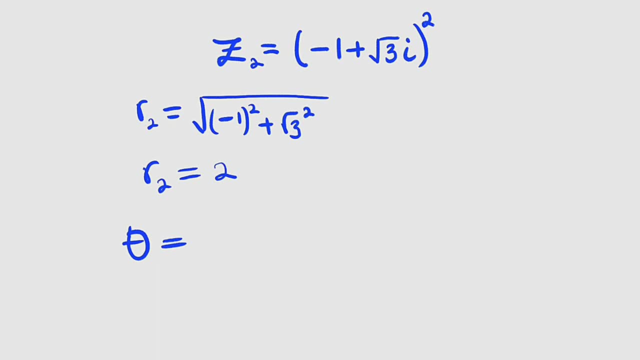 as reference. But whatever we obtain, we have to take it away from 180, which is pi. So this is pi minus tan inverse of what: The imaginary part, which is root 3, divided by the real part, which is 1.. 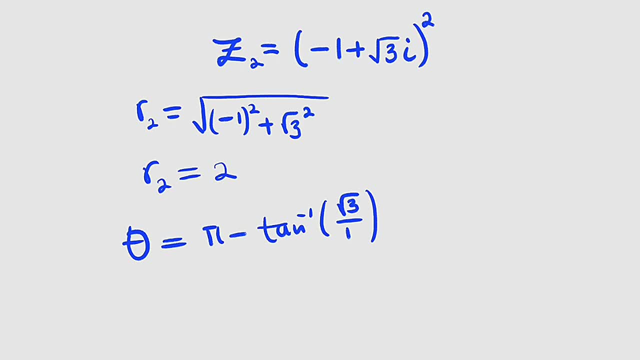 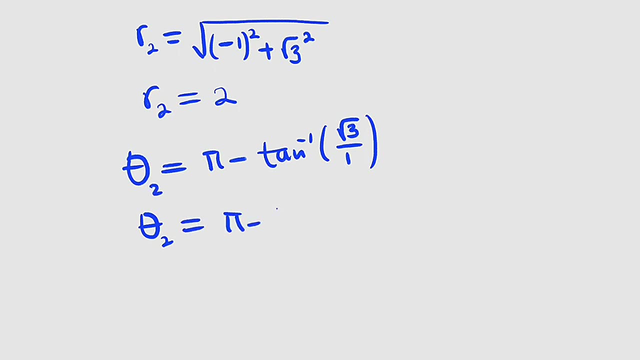 Root 3 divided by 1 is still root 3, and tan inverse of root 3 is pi divided by 3.. So our theta, which is theta 2, is equal to pi minus pi divided by 3,, which is 2pi divided by 3, right? Therefore, our theta 2 is equal to 2pi divided by 3.. 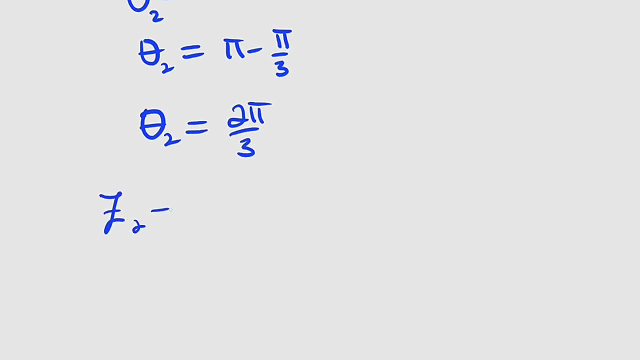 Therefore, that complex number- Z2, will be equal to R2, which we have as 2, multiplied by cosine of the angle, which is 2pi divided by 3, plus i sine of the same angle, 2pi divided by 3.. But remember that our complex number is to the second power. 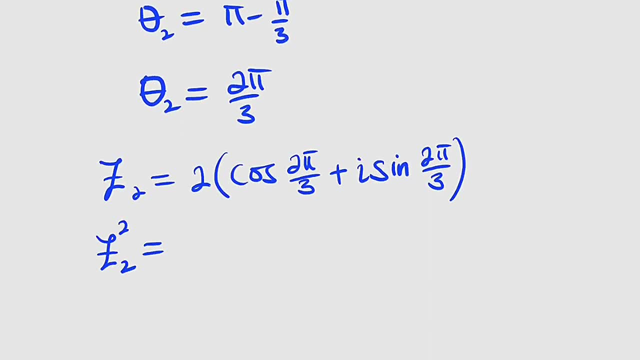 So Z2 to the power of 2 is equal to 2 to the power of 2.. Then multiply by cosine of what 2 multiplied by 2pi divided by 3.. Then plus i sine of what 2 multiplied by 2pi divided by 3.. 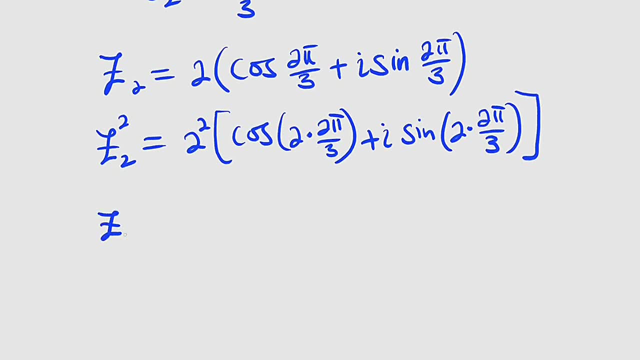 If you simplify this, Z2 to the power of 2 will be equal to 2 to the power of 2 is 4 multiplied by cosine of what 4pi divided by 3.. Then plus i sine of what 4 pi divided by 3.. So we are almost done. What do we need to do next? We 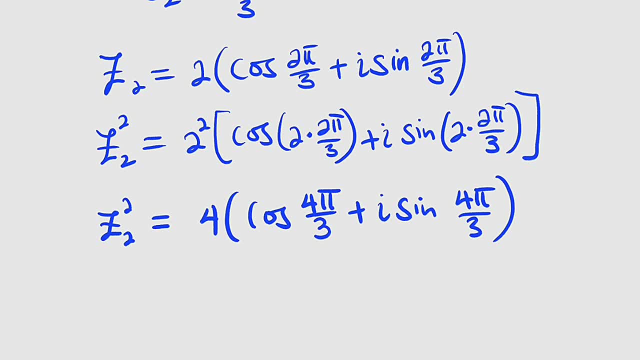 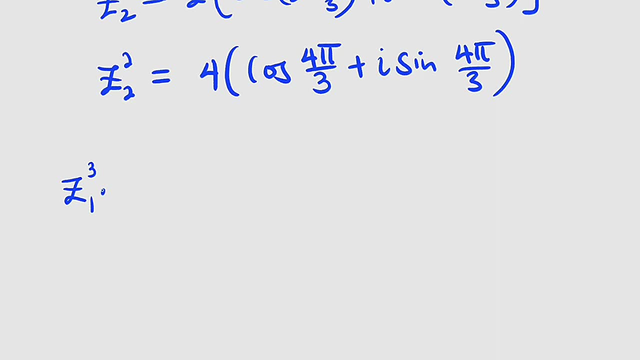 need to multiply z1 to the power of 3 by z2 to the power of 2.. So z1 to the power of 3 multiplied by z2 to the power of 2.. This is equal to r1 to the power of n multiplied. 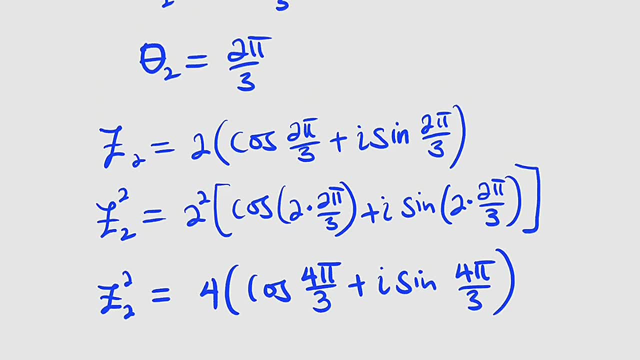 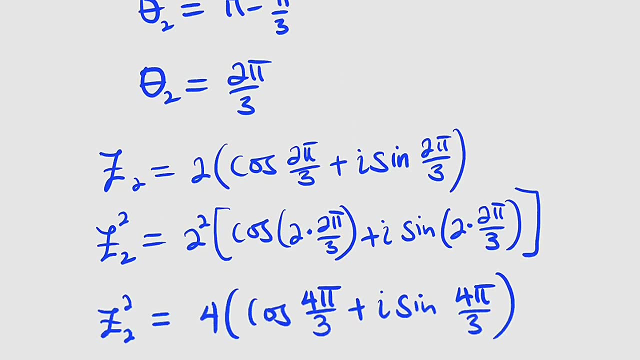 by r2 to the power of m right. And these are just the results. We have 64 for this one, which is our r2 to the power of 3.. And we have 4 here as our r2 to the power of m. 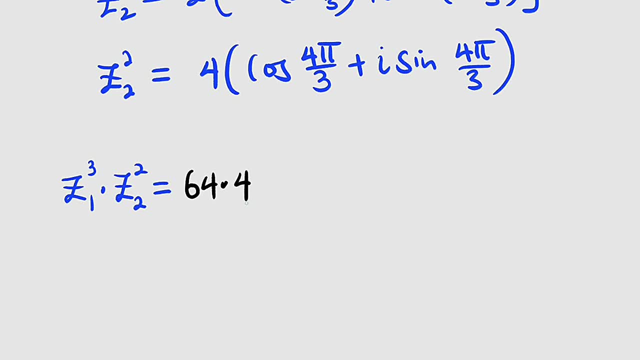 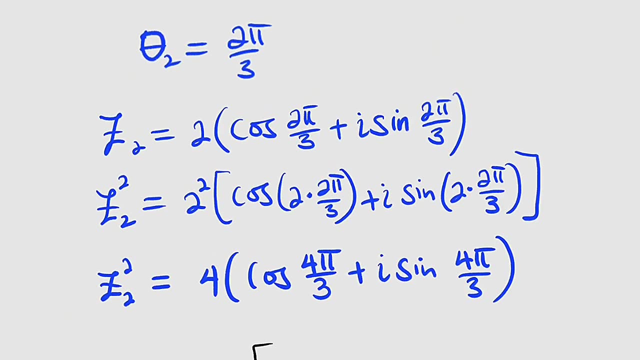 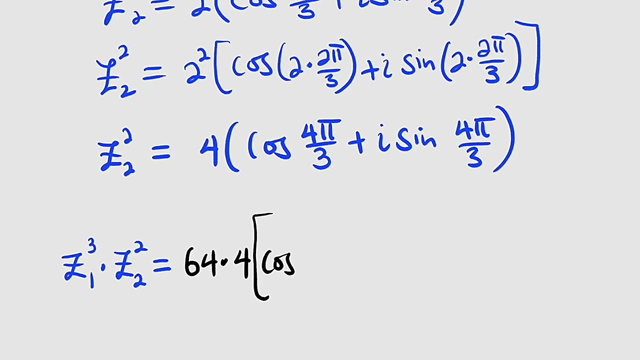 So we have 64 multiplied by 4.. Then inside we have cosine of what. We are going to add the arguments together. We have pi here. right, You can see we have pi here. But what do we have here? We have 4 pi divided by 3.. So we are going to add them together. 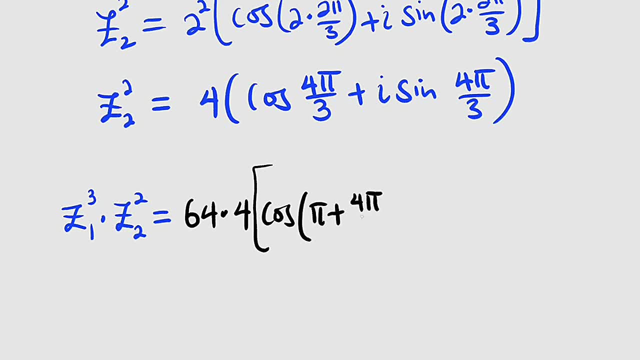 Pi plus 4 pi divided by 3.. Then plus i sine of the same thing, Pi plus 4 pi divided by 3.. We close. We have 64 multiplied by 4, which is 256.. So this is 256.. So this is 256. 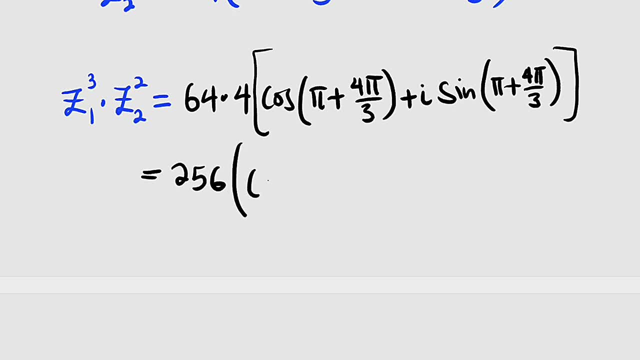 Multiply by cosine of what Pi plus 4 pi divided by 3,, which is 7 pi divided by 3 plus i sine of the same angle, 7 pi divided by 3.. All we need to find is cosine of this and. 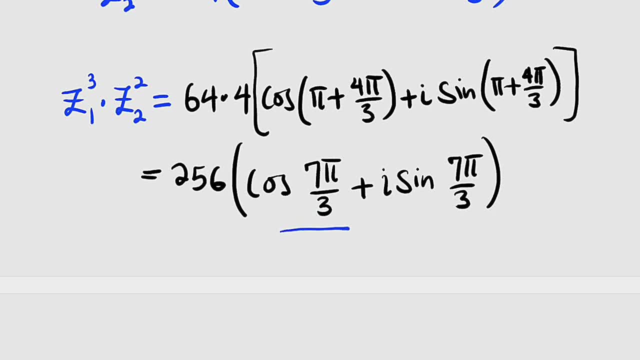 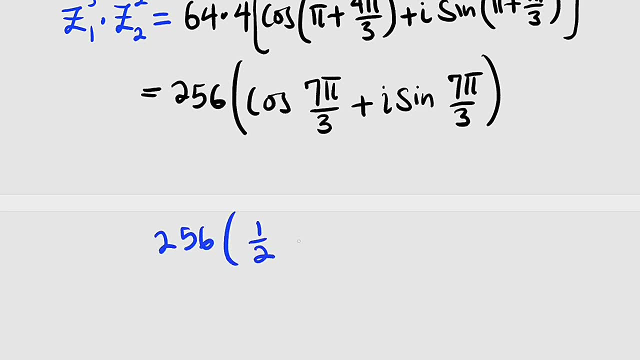 sine of this Cosine of 7 pi divided by 3 is 1 over 2.. So we have 2.. 5, 6 multiplied by 1 over 2, then plus i sine of this angle, 7 pi divided by 30 is root 30. 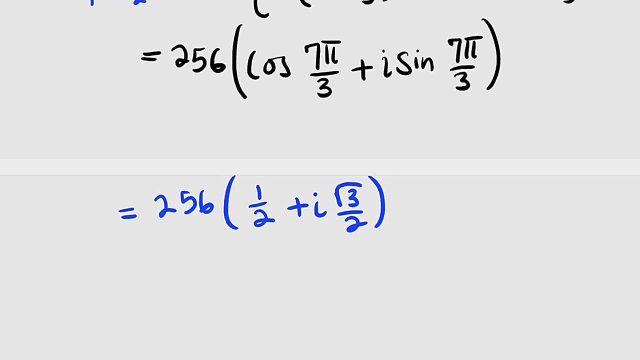 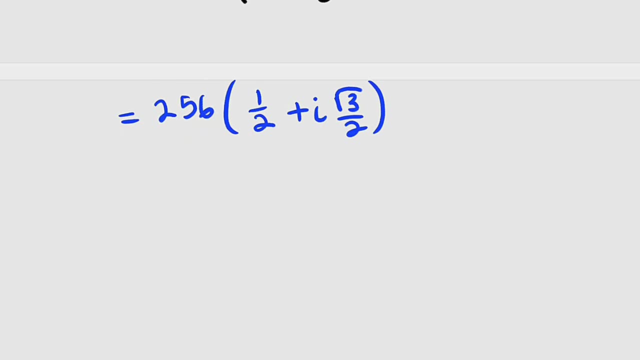 divided by 2, so let's distribute 256. multiplied by half is 128, so we have 128. 128 plus this, multiplied by this, will give us 128 root 30 i, 128 root 30 i, and hence this is just the result after multiplying these two complex numbers together. 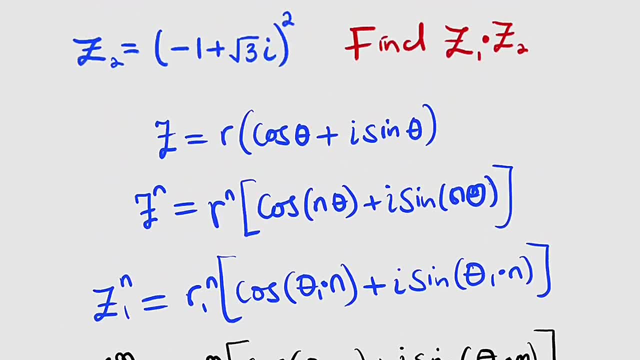 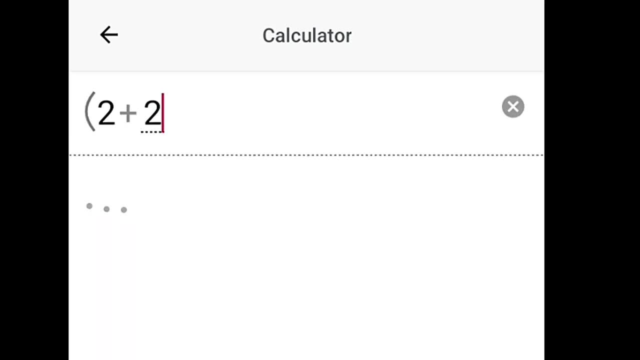 and i think i should use my calculator to prove this. so here is my calculator. our first complex number is 2 plus 2 root 3 i all to which power to the power of 30. and we want to multiply that with a complex number which is the second one, negative: 1 plus root 3 i to which power to the power of 2.